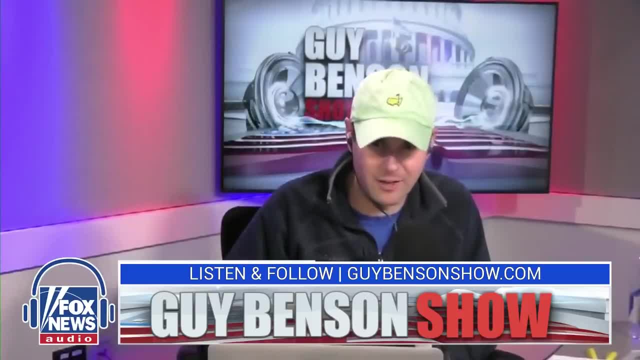 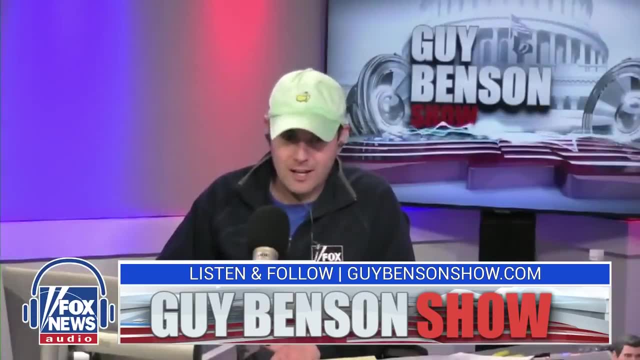 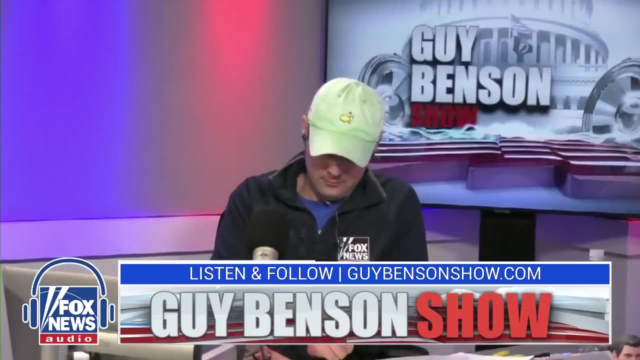 border As the border crisis czar doing a great job, obviously, And part of her very strange answer to that question with NBC News was this: cut 20.. Do you have any plans to visit the border At some point? you know we are going to the border, We've been to the border. 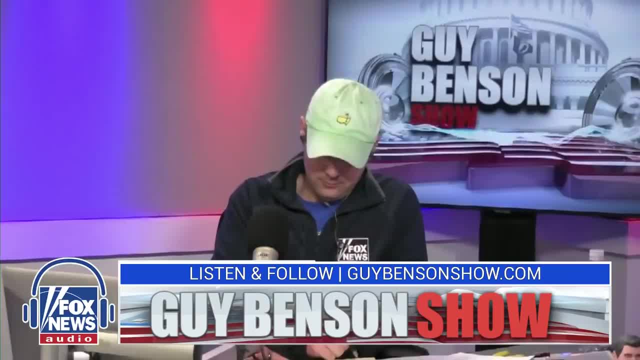 So this whole, this whole, this whole thing about the border, we've been to the border, We've been to the border, You haven't been to the border And I haven't been to Europe And I don't know. I don't understand the point that you're making. 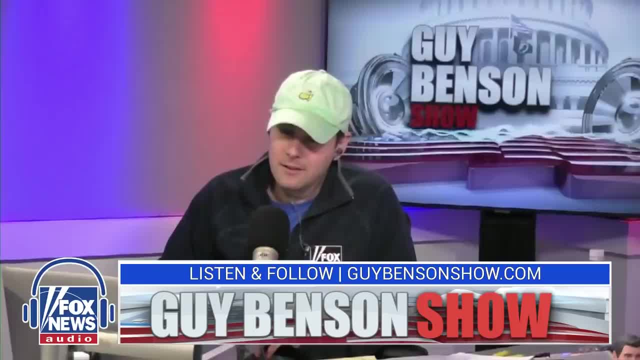 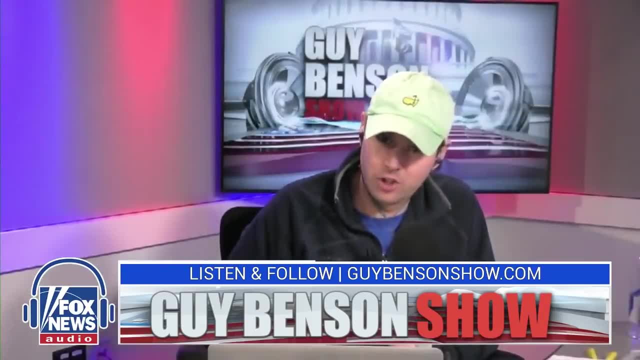 I'm not discounting the importance of the border. That was so strange, That was so awkward at the time And of course we got the laugh. We got the laugh in there at her little joke about having not gone to Europe. She said we've been to the border. 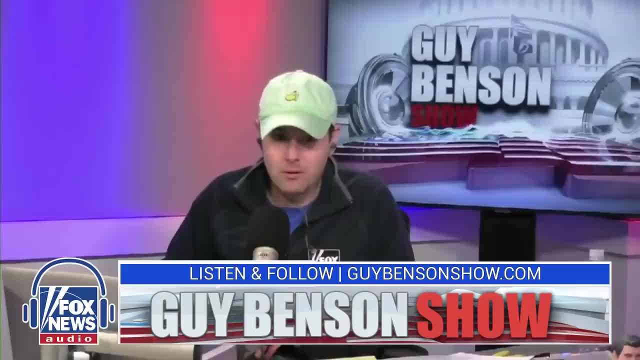 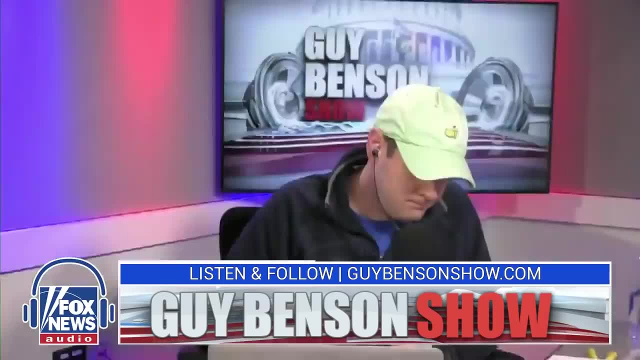 He said: well, you haven't. She's like, well, I haven't been to Europe. Well, now she's in Europe, So that must be very exciting for her. On Jimmy Kimmel's show last night, That's if you're unfamiliar. 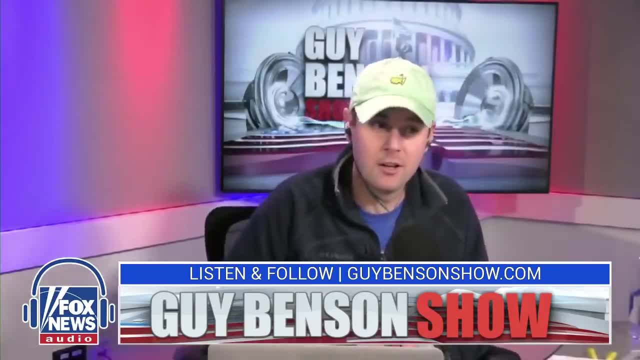 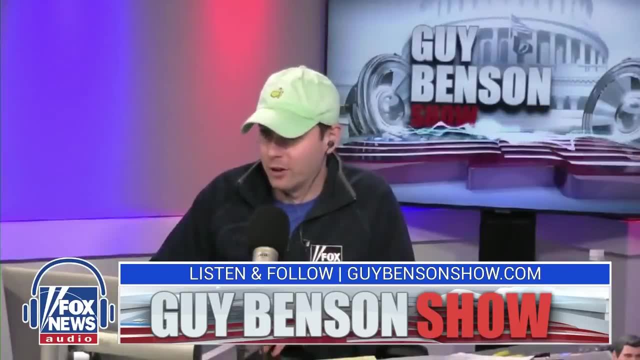 Jimmy Kimmel is a Democratic strategist and part-time comedian And he's got a show on one of the networks that loses to Greg Gutfeld every night. Gutfeld on cable, Kimmel on broadcast, And he loses every night to Greg Gutfeld, which is fun. 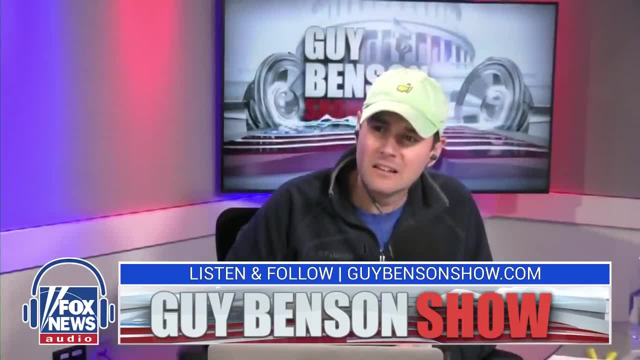 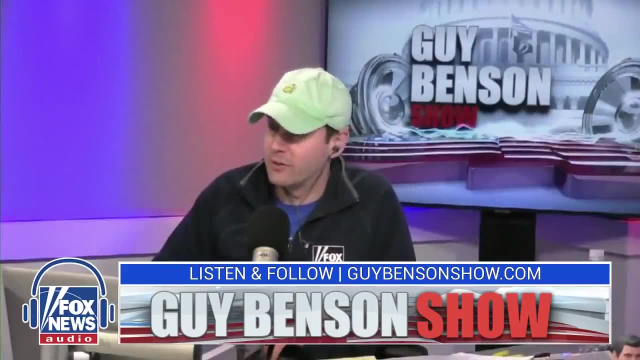 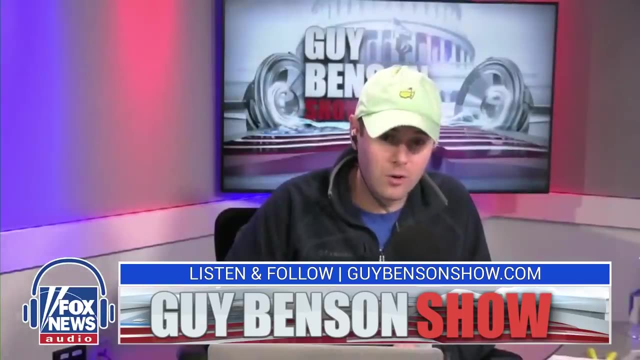 Jimmy Kimmel is a sort of kind of just sleazy, quasi-comedian guy who gets a lot of his talking points literally written for him by Chuck Schumer. That was actually revealed When he'll come out and do some of it. When he'll come out and do some of his little indignant monologues about Republicans, he gets his quote-unquote facts from Chuck Schumer's office. 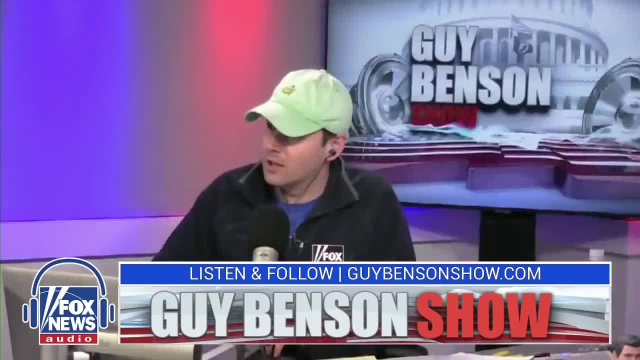 So he's a Democratic strategist, also a self-appointed pope. You know he wants everyone to take his moral decrees very seriously, As he should. I mean, he made his career as a guy who sat around drinking beer as women jumped on trampolines. 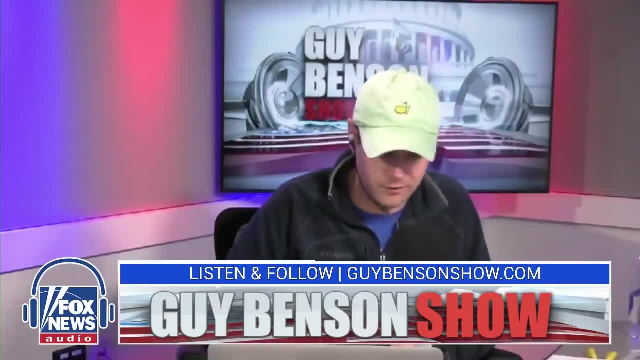 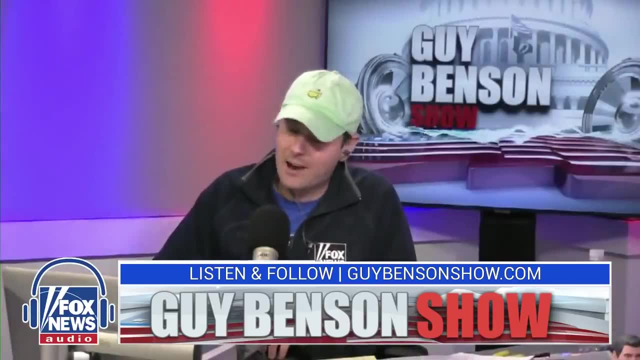 This is someone who can absolutely preach from on high to all of us. So this Democratic strategist and part-time comedian had some thoughts about Kamala Harris. It's been not a great couple of weeks on polling for President Biden or for Vice President Harris. 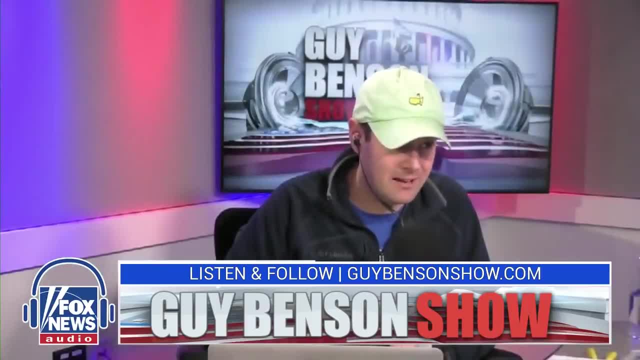 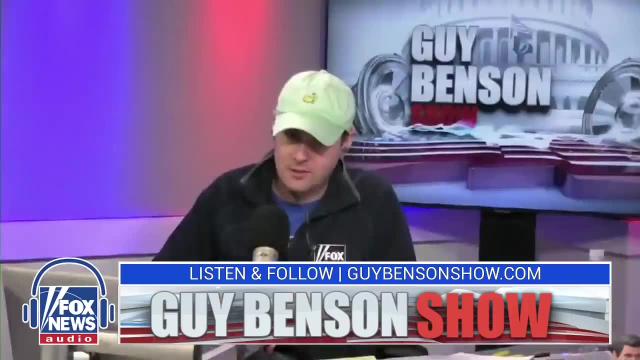 We talked about how Harris was just about as unpopular as Biden- slightly less popular, as a matter of fact, in this Suffolk USA Today poll- And Jimmy Kimmel was upset about this- a fellow Democrat, you know- is under attack, not garnering rave reviews from the American people. 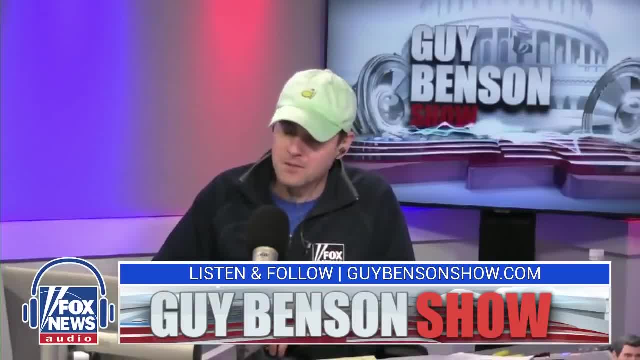 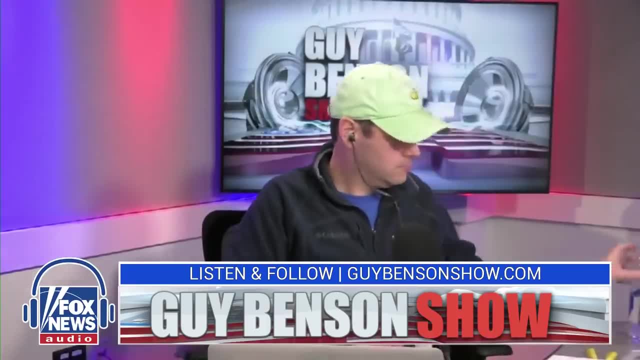 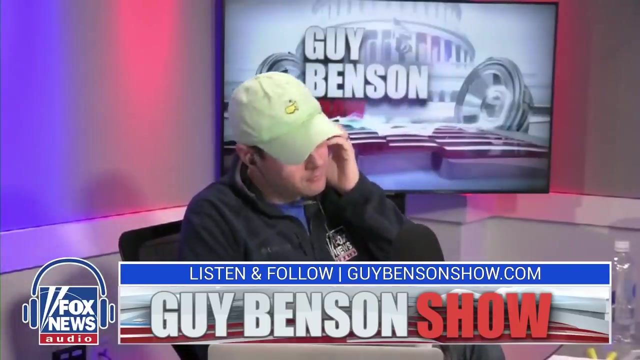 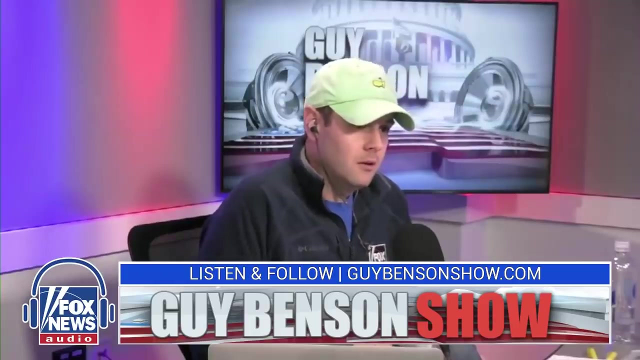 So Kimmel decided that Obviously the problem is the American people cut 14.. Yeah, And that's not enough for him. So I've got another thing to say. I don't know if you guys are aware of it. I mean, there's been a really nice 10% of voters who have been trying to be conscious of it. 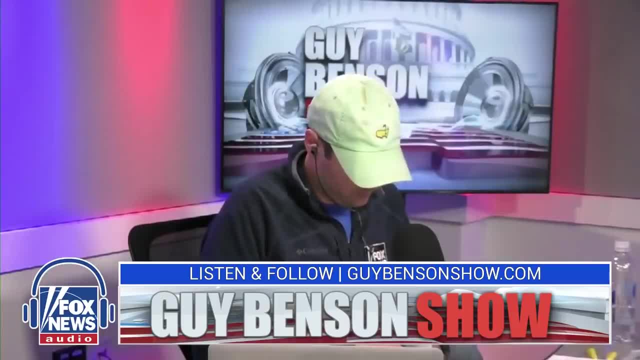 And I don't know if you guys are aware of it, but I think they don't want to come with right into it. I just don't have sexism or racism. I don't know how to explain it to you. Besides sexism and racism, the obvious reasons why her approval rating is so low: 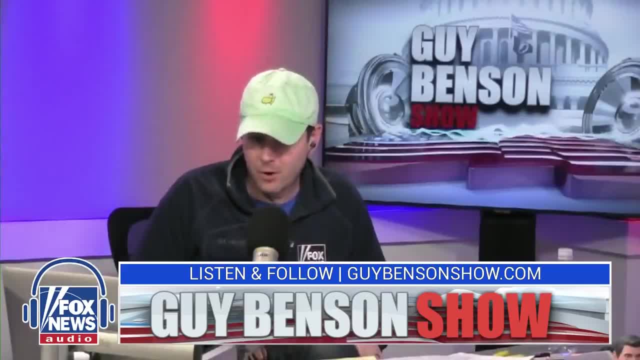 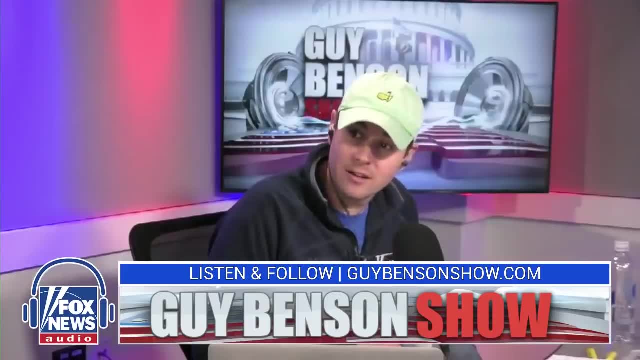 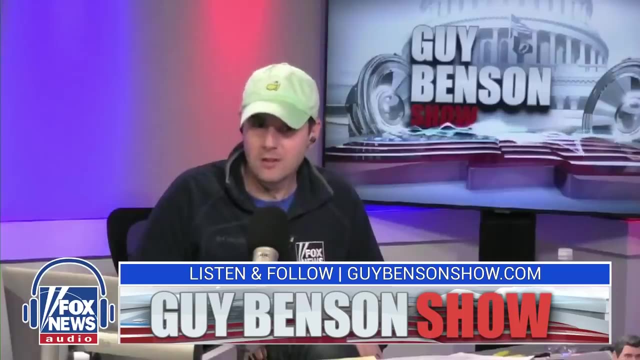 Well, you know she's at negative 23 in that poll, Underwater by 23 points. Biden is statistically the same, underwater by 21 points. Last time I checked, Joe Biden is a very white man. Now is it sexism and racism that explains his poor approval rating? or is that only for his similarly unpopular vice president, who he's put in charge of some big things like the border, which is a disaster? 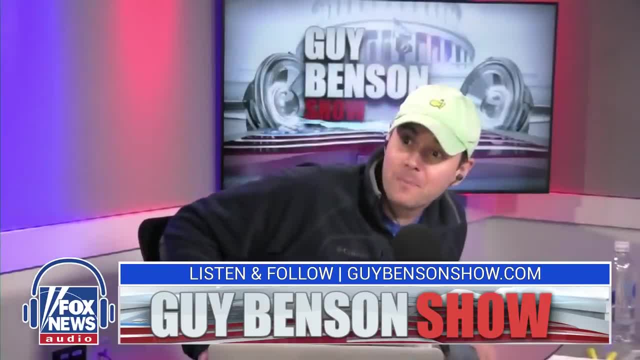 I know he's saying the vice president doesn't do anything. Maybe that's part of the problem: She's tasked with things and then doesn't do them or doesn't do. Maybe that's part of the problem: She's tasked with things and then doesn't do them or doesn't do. Well, it's sexism and racism. She's tasked with things and then doesn't do them or doesn't do Well. it's sexism and racism That explains why Harris is unpopular them or doesn't do Well. it's sexism and racism That explains why Harris is unpopular, But fill in the blank, for why? 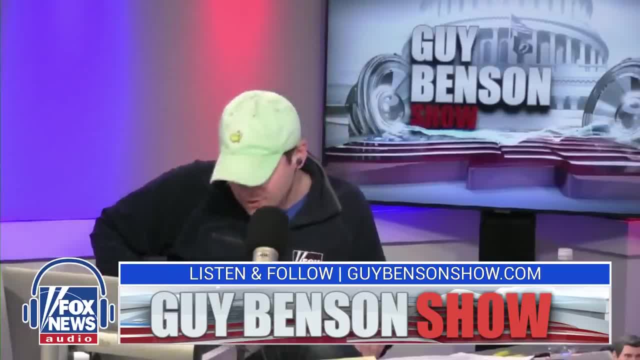 Well, it's sexism and racism That explains why Harris is unpopular, But fill in the blank for why Biden's unpopular. I'm sure it's. That explains why Harris is unpopular, But fill in the blank for why Biden's unpopular. I'm sure it's probably more of the same. 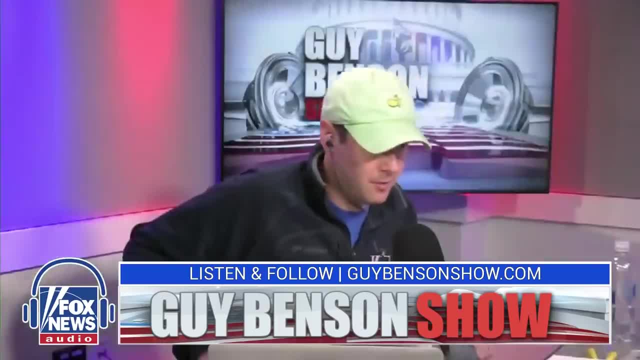 But fill in the blank. for why Biden's unpopular? I'm sure it's probably more of the same: Because they see sexism and. But fill in the blank. for why Biden's unpopular? I'm sure it's probably more of the same: Because they see sexism and racism as a built-in excuse, always and forever. 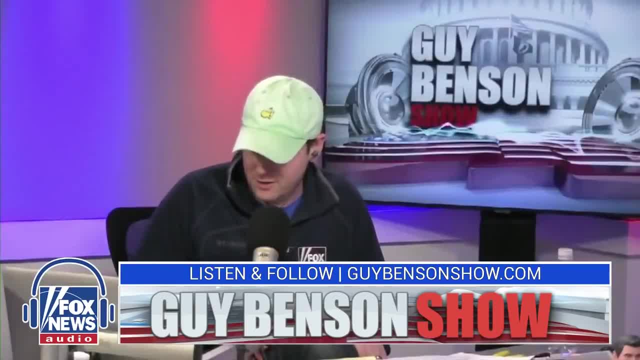 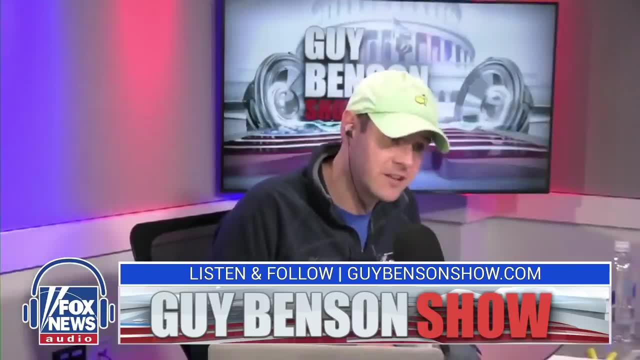 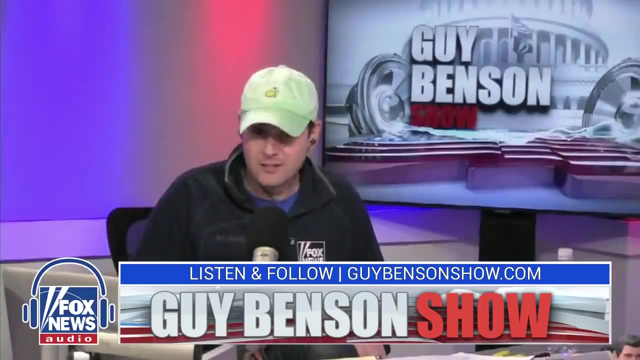 It couldn't possibly be the failures of the administration and the leaders of that administration and the two most high-ranking government officials in the entire United States of America. I know It's a big, difficult thought for Jimmy, So he's got his answer there. 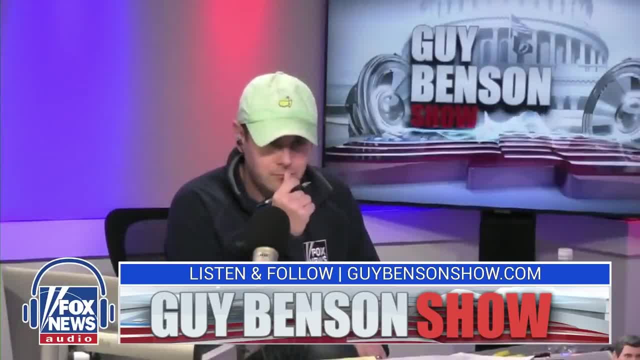 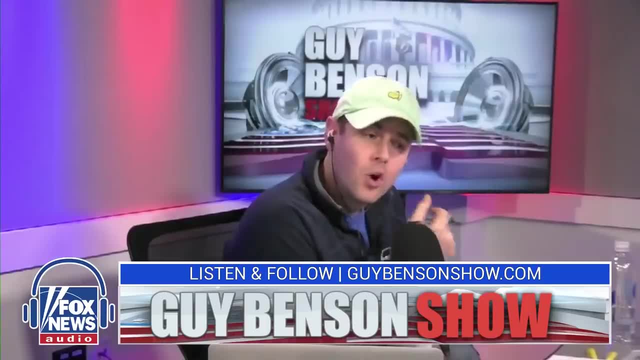 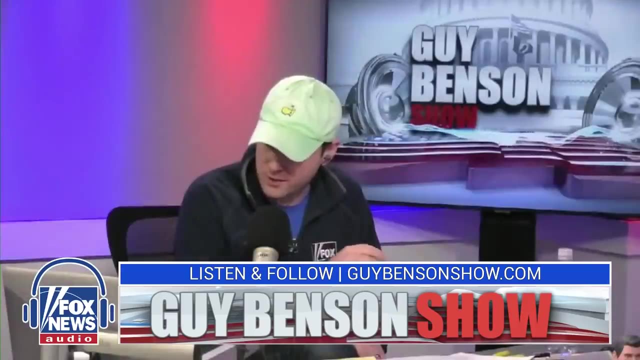 It's sexism and racism. I actually do have a thought, though kind of like a follow-up question for Jimbo here, which is: why is it that Kamala Harris, when she was running for president, remember she called Joe Biden a racist during that campaign? 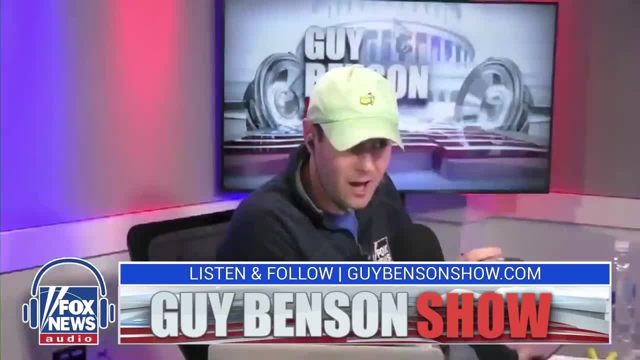 Remember that one. She was running for president. She wanted his job, not her current job. She was such a bad candidate. She was such a bad candidate for president that she didn't even survive. The candidacy did not even survive to Iowa. 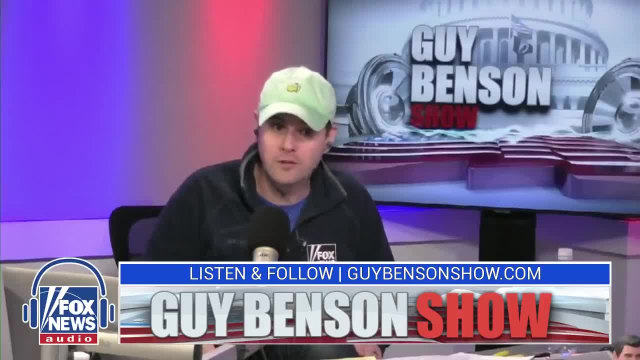 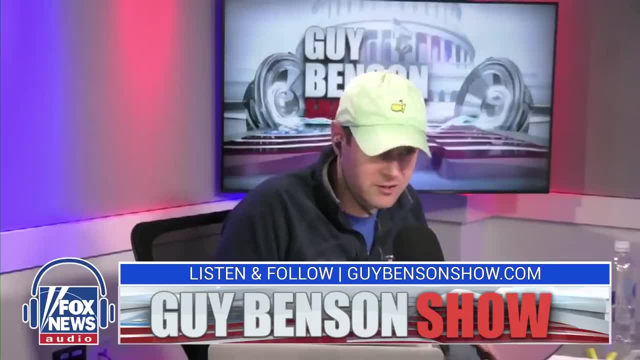 She dropped out before a single primary or caucus voter even showed up, And I know this might be difficult for Jimmy to remember if he even knows this stuff. Maybe you get a little quick refresher or tutorial from Chuck Schumer. But that was a Democratic primary. 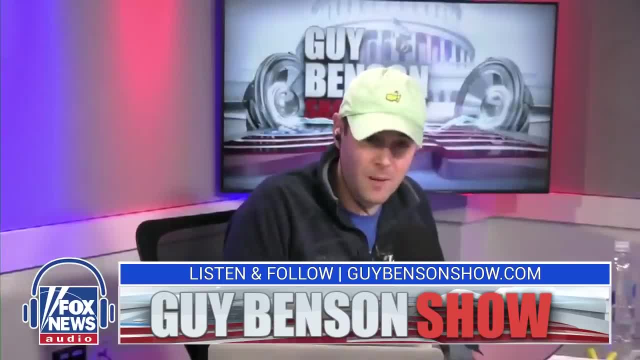 That was all his team, their side, And by his team I mean, you know the Democrats, The side. you know that he embodied, for example, when he lost to Ted Cruz in a one-on-one basketball game, Something he should never live down. 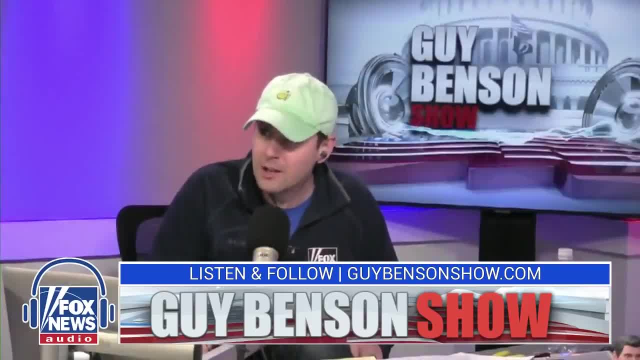 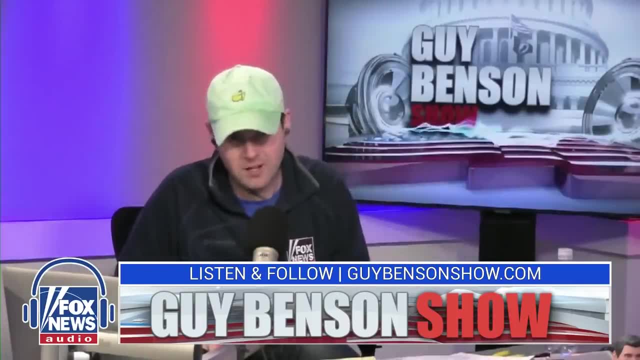 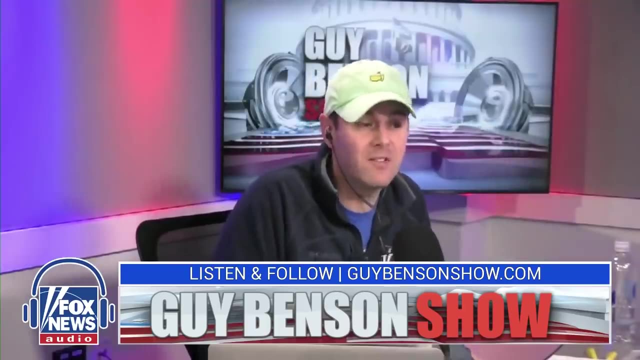 Hilarious. It was his team, his party, the enlightened, non-racist misogynists supposedly in their party, who were so unimpressed by Kamala Harris that they rejected her forcefully enough in the polls that she didn't even bother to come to Iowa to get humiliated and lose badly by her own. 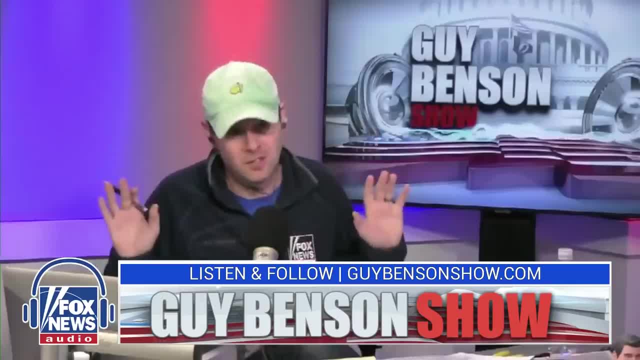 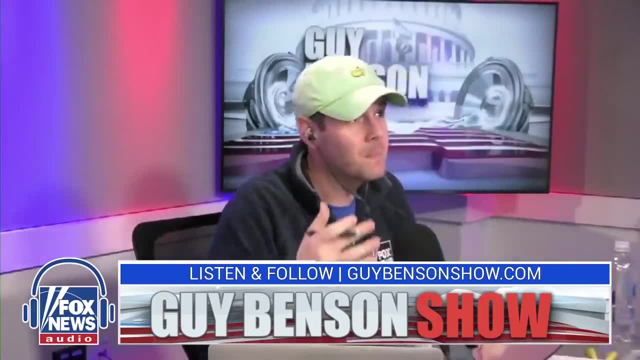 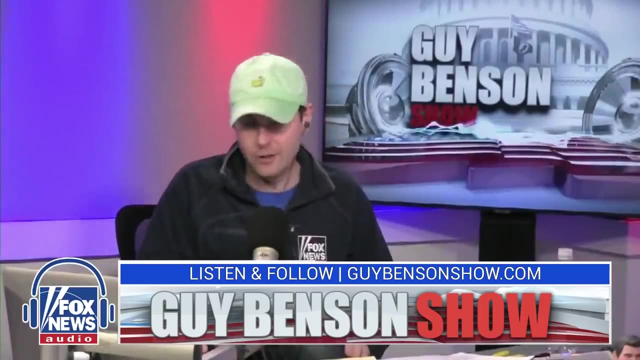 So this is not the kind of thing that was done, And this was a good thing for judge Kemp. Use that as excuse, because it's an assignment to vote for the next president, of course, in the item of your choice on the majority vote besides voters. 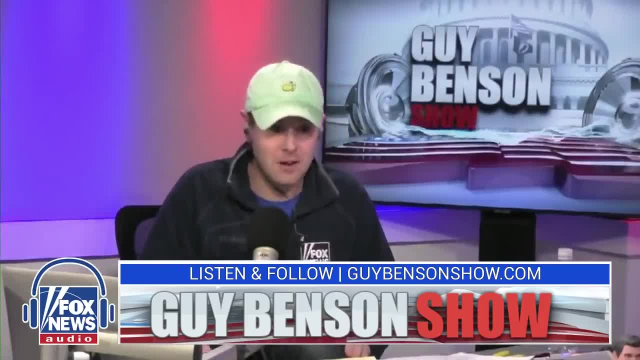 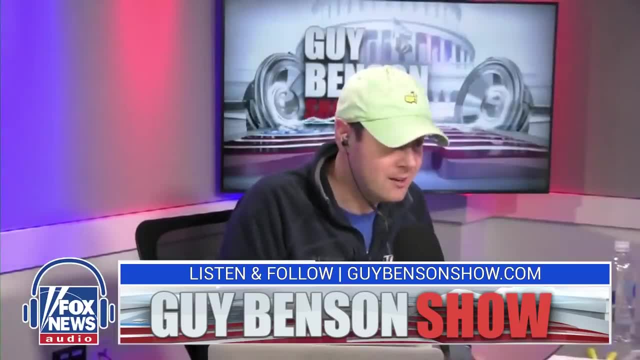 Maybe that's also sexism and racism, Jimmy, I don't know, But the proof was in the pudding In the Democratic primary. So my theory is maybe her approval rating is a tied to the flailing president, Tied to the failing administration.